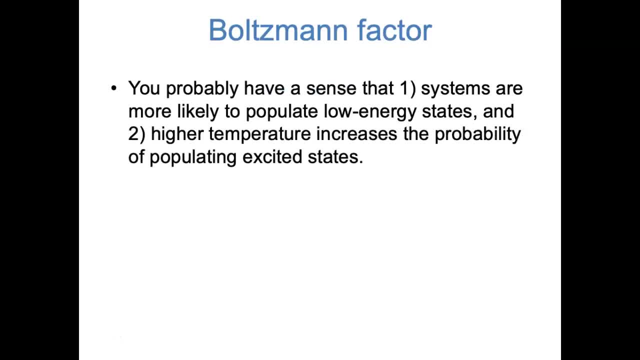 Even though we haven't yet quantitatively talked about temperature, you probably have an intuitive sense of certain things. You probably know, for example, that systems are more likely to populate low energy states. We often talk about lower energy states as being more stable, and you've also seen things like the Aufbau principle, where electrons 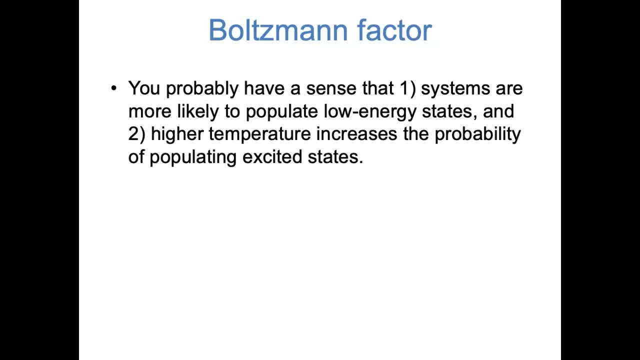 tend to populate lower states. You probably also have a sense that higher temperatures tend to increase the probability of populating excited states. You know, for example, that higher temperatures tend to make reactions more likely to happen to cross over transition state barriers. 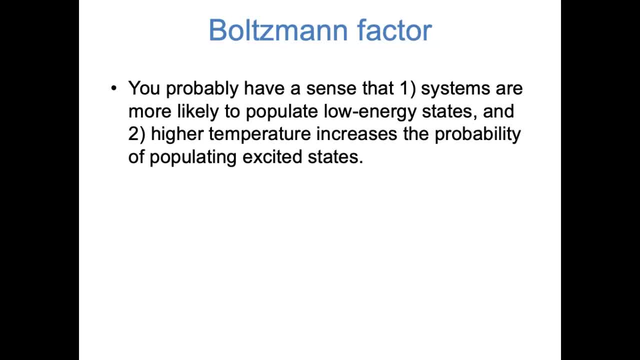 But what we're going to do now is to quantify these ideas. This expression is the definition of a Boltzmann factor which may be the most important concept of quantum mechanics. P with a subscript j is the probability that some energy state j will be occupied. The 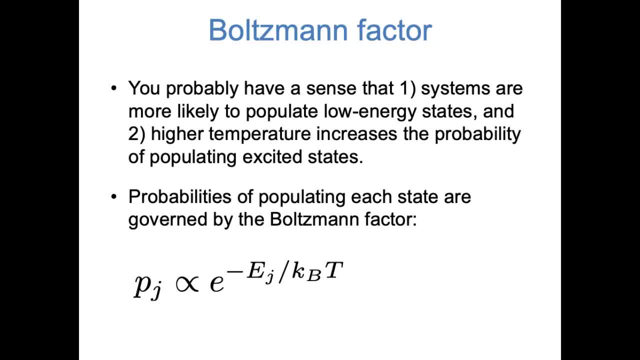 symbol next to it means that it's proportional to and the expression on the right is the Boltzmann factor: an exponential e to the negative energy of state j divided by kB T. First a little terminology: kB is the Boltzmann constant. You've probably seen the gas constant. 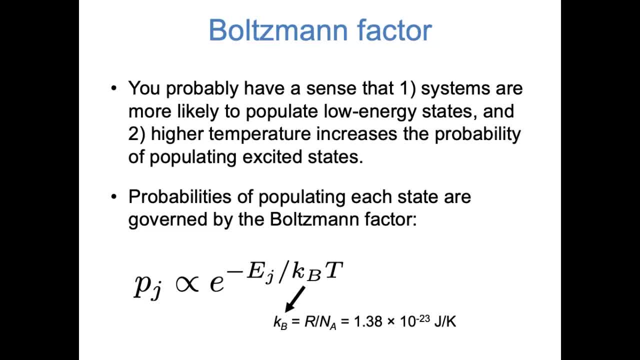 capital R, And the Boltzmann constant is just the single particle version of the gas constant. It's R divided by Avogadro's number, which in SI units is equal to 1.38 times 10, to the negative 23 joules per kelvin. 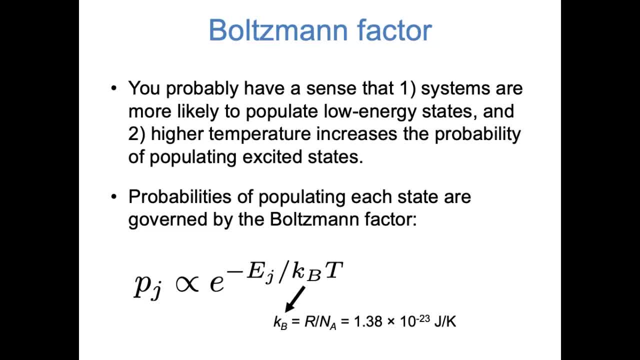 So if you look at the units in that exponent, if we use an energy in joules, a Boltzmann constant in joules per kelvin and a temperature in kelvin, then all of the units in the exponent will cancel out and the exponent will be unitless. 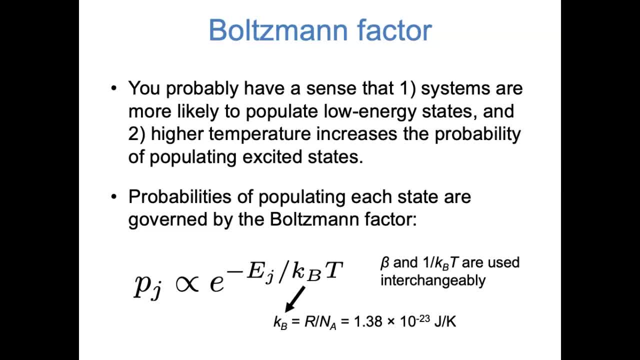 Throughout statistical mechanics. we'll often see a lot of kB T's in the denominator, So you'll sometimes see 1 over kB T written as the Greek letter beta in shorthand. So a Boltzmann factor can alternatively be written as e to the minus beta times, energy. 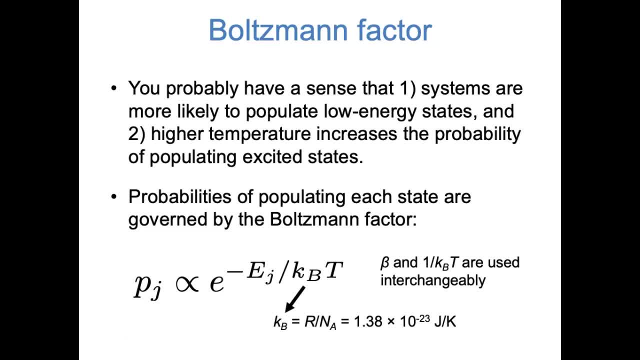 If you look at this whole expression, you'll notice that as the energy gets higher, the exponent becomes a larger negative number, and so, as the energy gets higher, the probability of occupying a state gets smaller. That makes sense. As we said, lower energy states are more likely to be occupied than higher energy states. 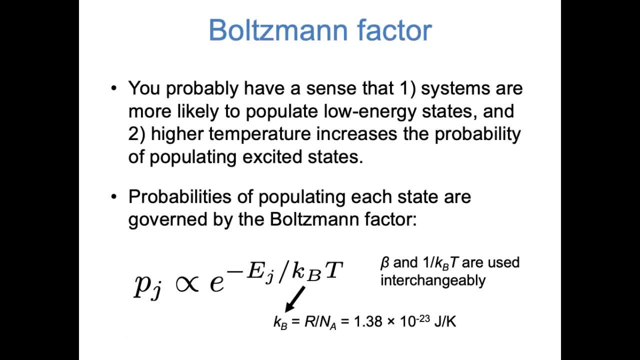 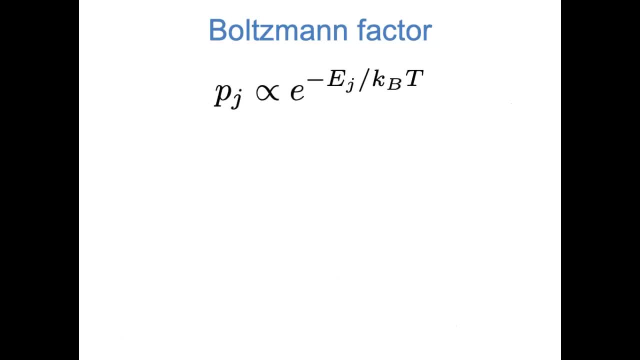 Also notice that as the energy gets higher, probability doesn't just get lower, it gets lower really quickly. It goes as an exponential. I'd like to say a couple more things about this expression to help us wrap our minds around the idea of Boltzmann factors. 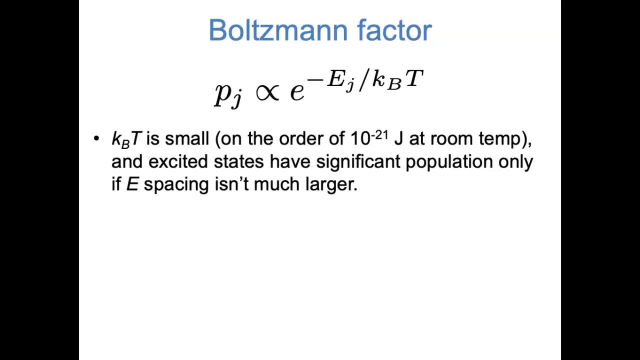 First of all, numerically, kB T is really small. We saw that kB is on the order of 1 over kB T. We saw that kB is on the order of 10 to the minus 23 joules per kelvin, And most of the time we're thinking about temperatures that are in the hundreds of kelvin. 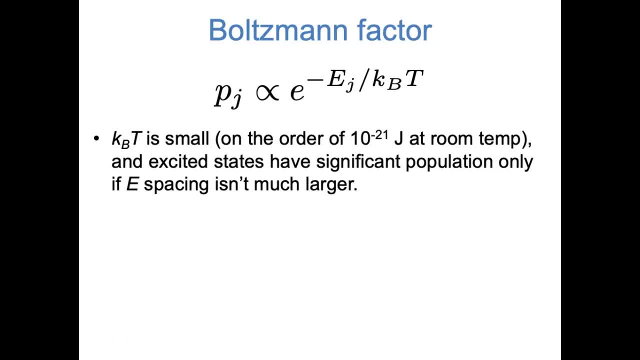 So around room temperature, kB times T is on the order of 10 to the minus 21 joules. The upshot of that is that if the energy levels of an atom or molecule are spaced much farther apart than 10 to the minus 21 joules, then really only the ground state will have significant. 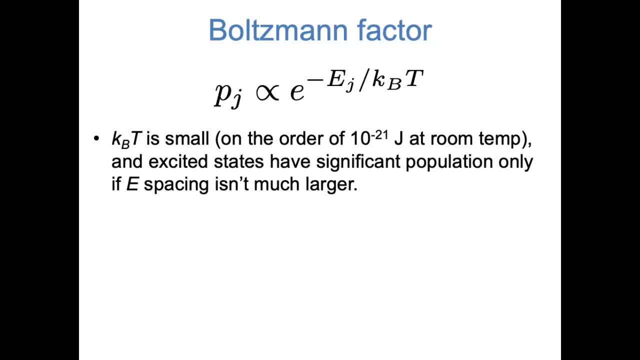 occupation. It's only when the energy levels of an atom or molecule are really close together, on the order of 10 to the minus 21 joules, that we see significant population of the excited states. Also, remember that our absolute definition of energy is arbitrary and it's really only 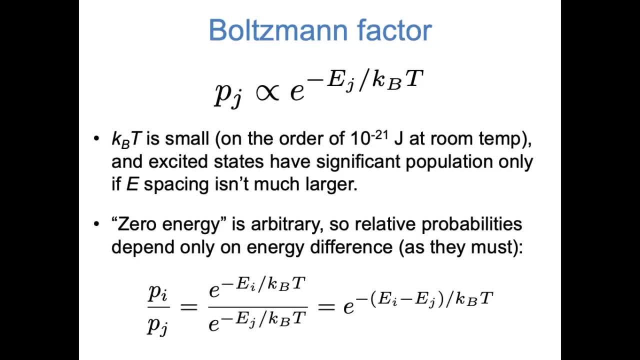 differences in energy that are meaningful. That means that the relative probabilities of two states being occupied must only depend on the difference in energy, and we can show that If we look at the probabilities of two states being occupied, Pi divided by Pj can be written. 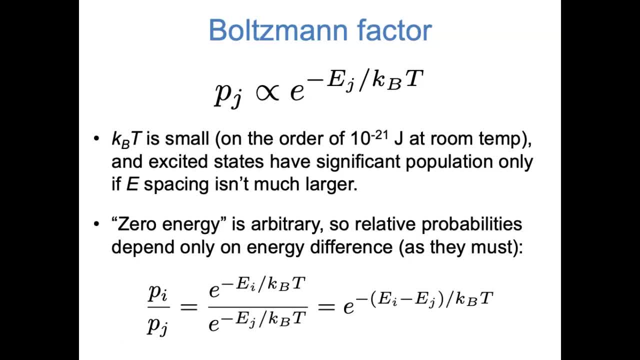 as a quotient of Boltzmann factors And if we remember our exponent rules, if we divide one exponential by another, we subtract the two exponents and we can see that the quotient of those two probabilities does in fact depend only on the difference between the energies. 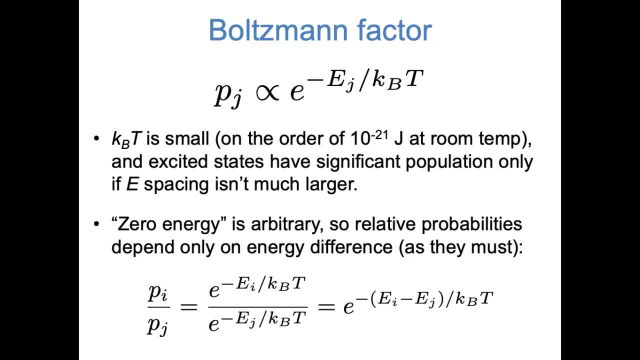 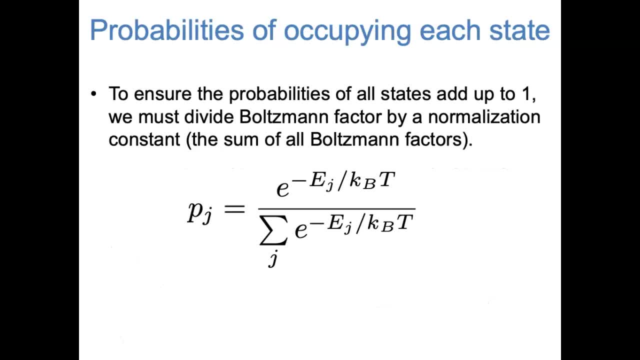 That's something that had to be true, because our definition of zero energy was arbitrary. So far, we've said that the probability that a state has two states being occupied is only proportional to the Boltzmann factor, But we haven't yet said what the probability is equal to, and that's something that we'll 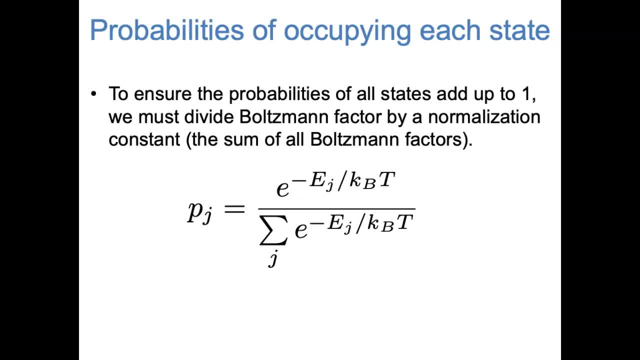 often want to calculate To figure out what a probability is equal to. we basically just need to ensure that the probabilities of all possible outcomes add up to one, because that's how probabilities work. So in order to find a probability Pj, we need to take the corresponding Boltzmann factor. 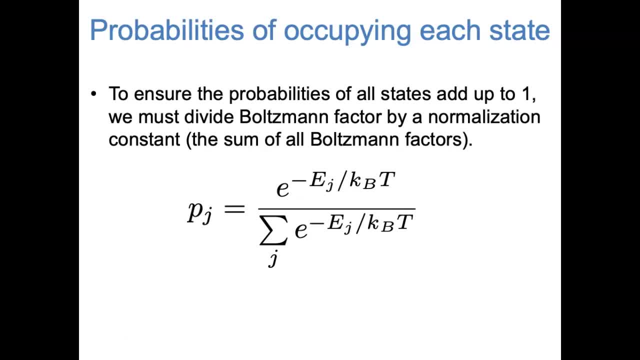 and divide it by a normalization constant, which is basically just a constant, And that's just a sum of all of the possible Boltzmann factors. For example, if an electron has three possible states that it can be in, the normalization constant is just the sum of the Boltzmann factors for those three states. 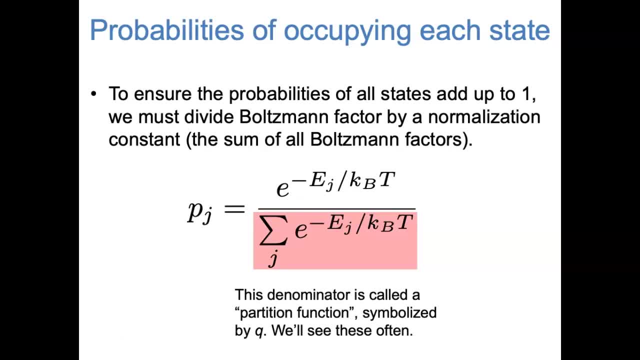 In statistical mechanics we actually give this normalization constant a name. It's called the partition function. It may seem a little bit silly at first that we give a name to this normalization constant, but it turns out that this partition function is actually very powerful and it can tell. 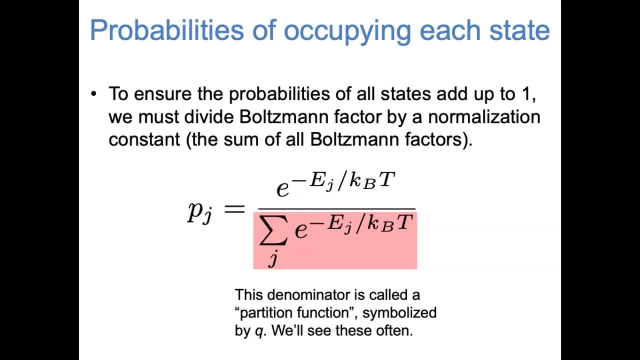 us a lot just by itself. So for now, just be aware that this is called the partition function, it's often symbolized by the letter Q and that we'll be seeing a lot of this in the upcoming videos. For the remainder of this video, I'd like to work through an extended example where 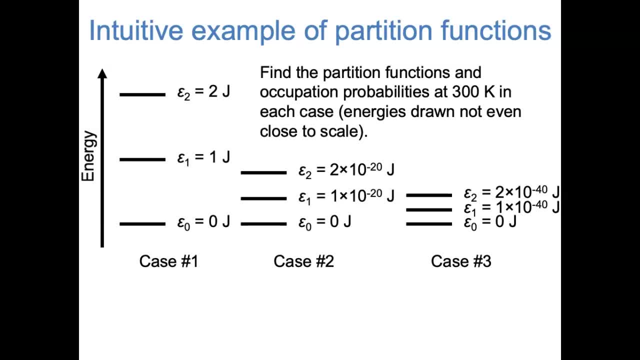 we try to make some numerical sense of Boltzmann factors and partition functions and what they mean. We're going to look at a particle that has three possible energy states that we'll call epsilon 0,, epsilon 1, and epsilon 2.. 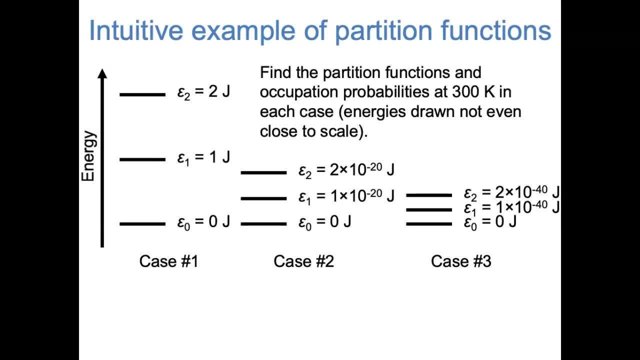 It doesn't even really matter whether that particle is an electron or an atom or a molecule. you can just think of it as any particle that has three possible energy states. And we're going to look at three different cases. In case number one, the three energy states are very far apart. 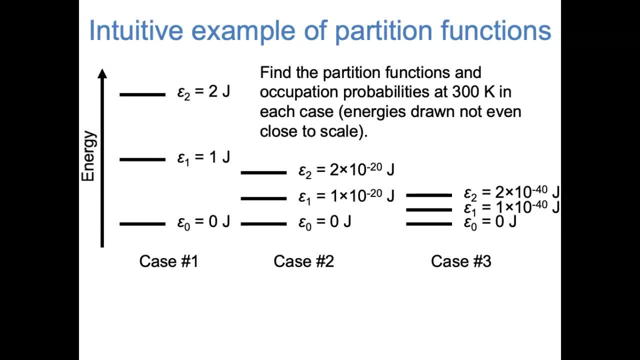 They're at 0 joules, 1 joule and 2 joules. In case number two, the energy states are spaced by 10 to the minus 20 joules, and in case number three, the energy states are spaced by 10 to the minus 40 joules. 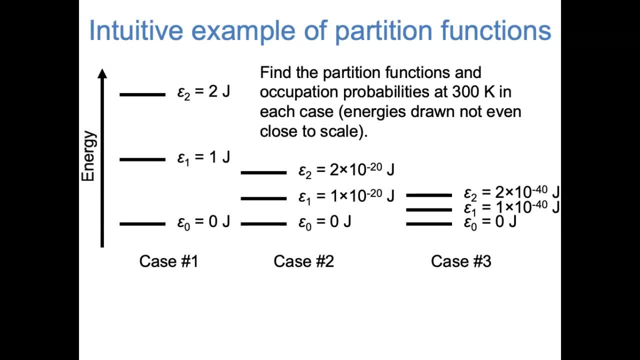 Notice that the way I've drawn these three cases are not even close to scale. From one case to the next. the energy spacing is different by many orders of magnitude and that's not what I've drawn. I've just tried to make it clear that the energy spacing goes from big to medium to small. 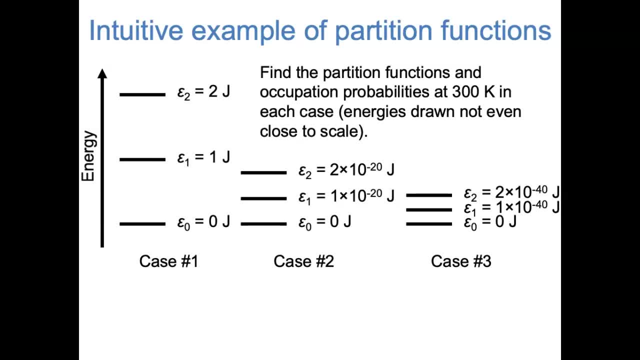 What we're going to do is, at 300 Kelvin at room temperature, we're going to find the partition functions for each of these three cases and the probability that each of the three energy states is occupied Before we calculate any numbers here. 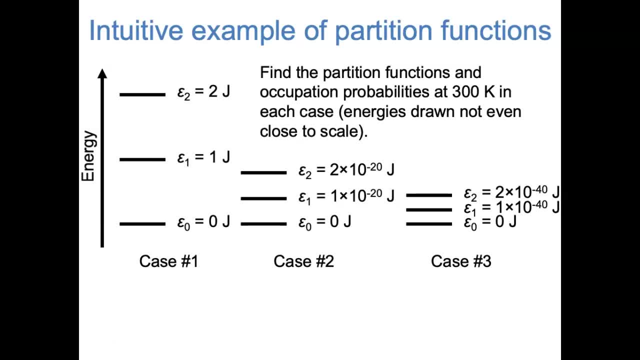 I'd like you to take a few seconds to think about how you expect these cases to come out, specifically in terms of the occupation probabilities In cases one through three. do you expect it to mainly be one state that's occupied? Do you expect all three states to be equally occupied? 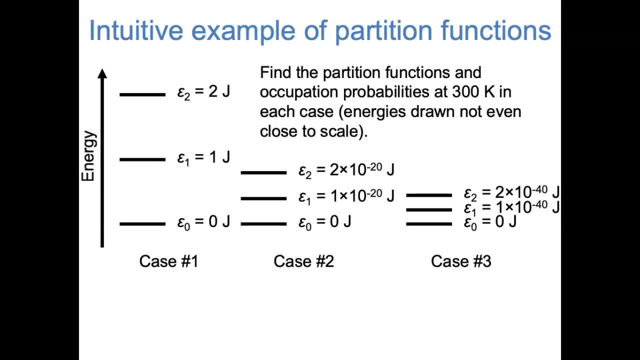 How do you think the relative occupations will turn out? I'll give you a few seconds to think about that and I suggest hitting pause to take some more time In case one. the energy states are spaced really far apart relative to kB T. 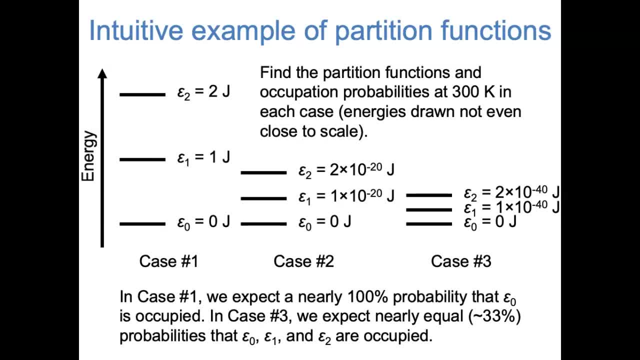 That means that in case one, we expect a nearly 100% chance that the ground state, epsilon zero, is occupied. In case three, the three energy states are so close together that they might as well be equal. That means we expect those three energy states to be nearly equally occupied. 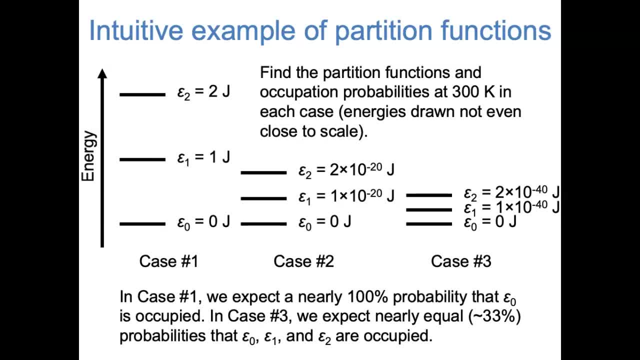 with about one-third occupation probability, And case two is somewhere in between. The energy spacing is pretty similar to kB T, which means that the ground state will be more occupied than the others, but we expect all three states to have some probability of being occupied. 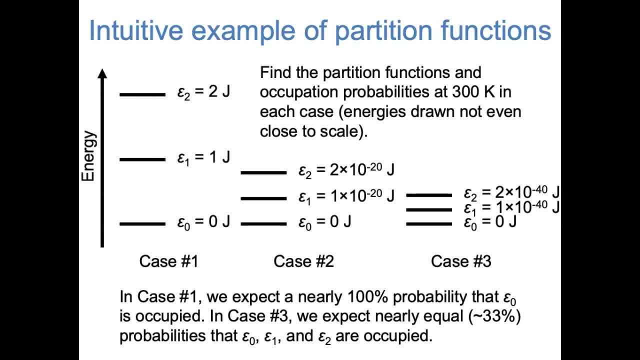 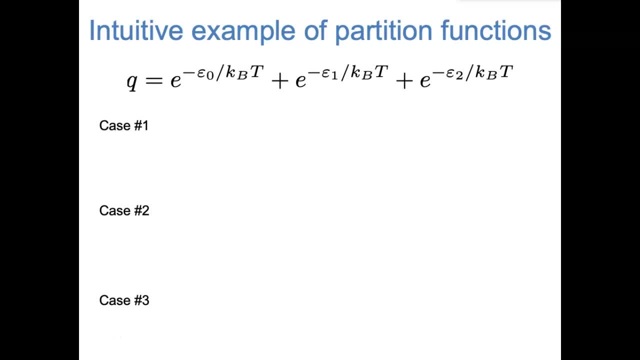 So that's what we expect, and we should try to keep that in mind as we work through the numbers. on the next slide The general form of the partition function is shown here. Q equals the sum of the three Boltzmann factors corresponding to each of the three energy states. 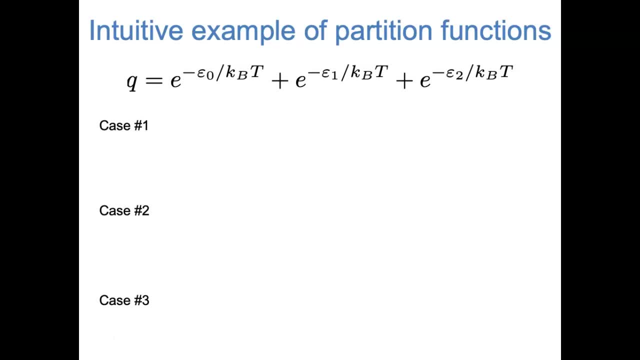 To find the Boltzmann factors and partition functions for each case, we just need to plug in the corresponding values of epsilon and T. We'll start with case number one. In case one and for all the cases, epsilon zero equals zero. 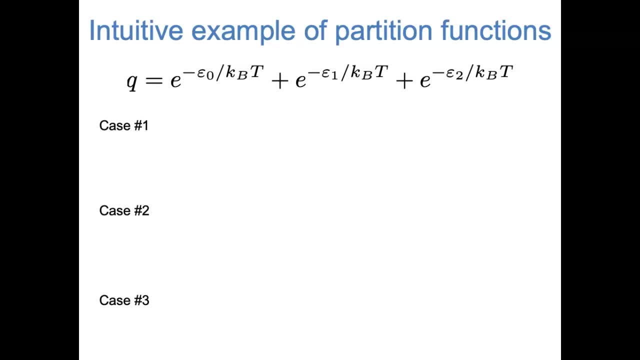 so the first term in each partition function is going to be e to the negative zero, which is just one. In case one, the two excited state energies, epsilon one and epsilon two, are both really high. so that means the second and third terms in the partition function. 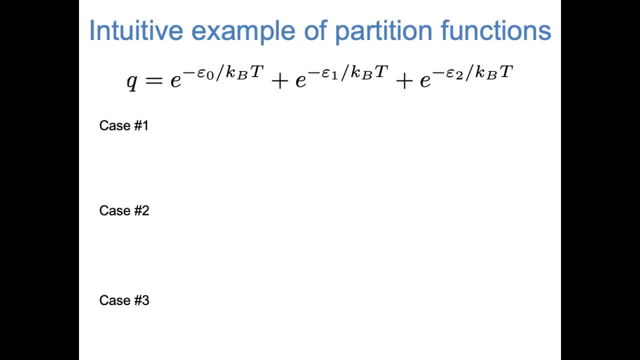 are going to be e raised to the power of a negative, really really large number And e to a negative, really really large number approaches zero. That means the partition function for case one is going to be one plus numbers approaching zero, which equals one. 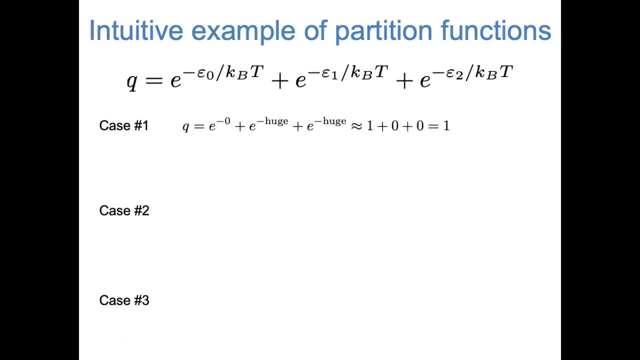 And then if we want to find the probability that each individual energy state is occupied, we just need to take each Boltzmann factor and divide it by the partition function. So the probability that the ground state is occupied is one divided by one. 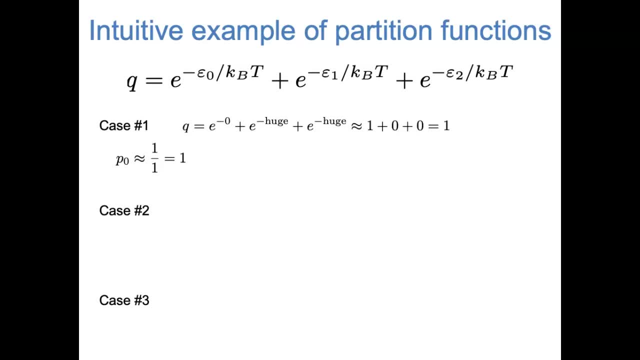 which is one. That's what we expected: a hundred percent probability that the ground state is occupied in this case, And then the probability that each of the excited states are occupied is just the Boltzmann factor, which approaches zero divided by the partition function. 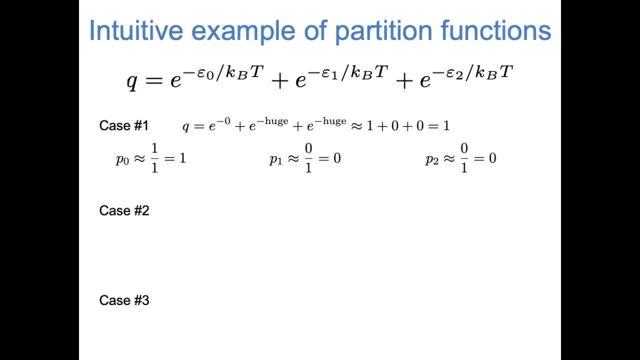 So those probabilities approach zero. That's all what we expected At the other end of the spectrum is case number three. again, the first term of the partition function equals one, because it's just e- to the negative zero. But in case three, 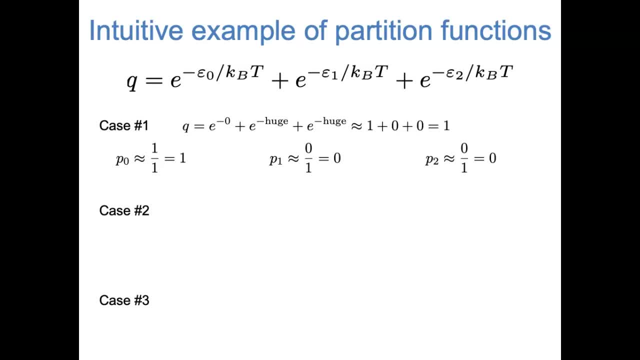 the excited state energies are also really, really small compared to kB T. So the second and third terms of the partition function are e raised to the power of negative, really, really small numbers, And again those approach e to the zero, which is one. 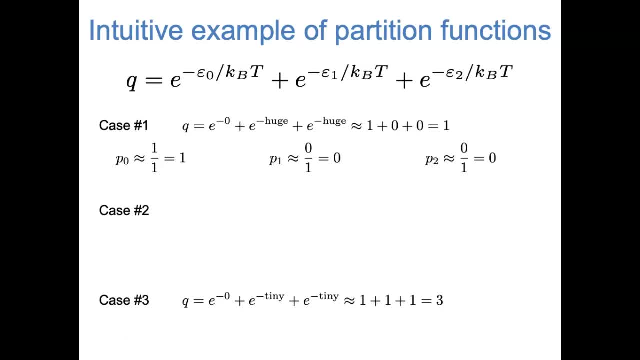 So in this case the partition function looks like this: It's the sum of three terms that all approach one, so the partition function approaches three. The probabilities that each state is occupied is just each individual Boltzmann factor divided by the partition function. 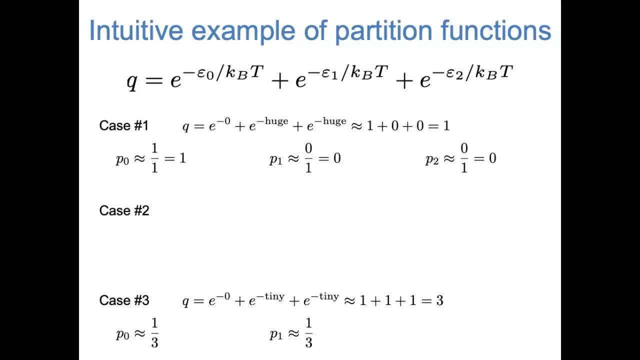 and each of those is going to approach one over three. So, as we expected, if the three energy states are infinitesimally close together, the probabilities of being occupied all approach one. third Case, number two, is the intermediate case. Again, the first term of the partition function equals one. 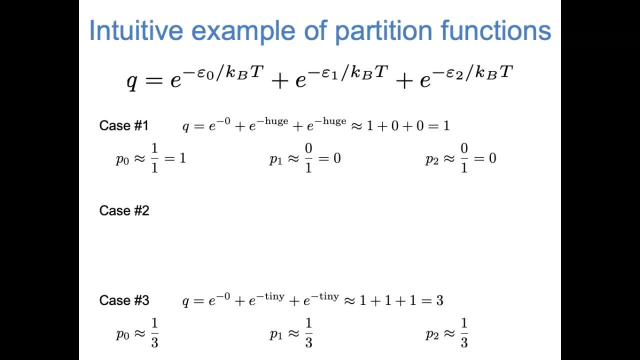 because it's just e to the zero. But for the second and third terms we actually need to plug in the excited state, energies and the temperature. It comes out like this: The first term is one and the second and third terms get smaller and smaller. 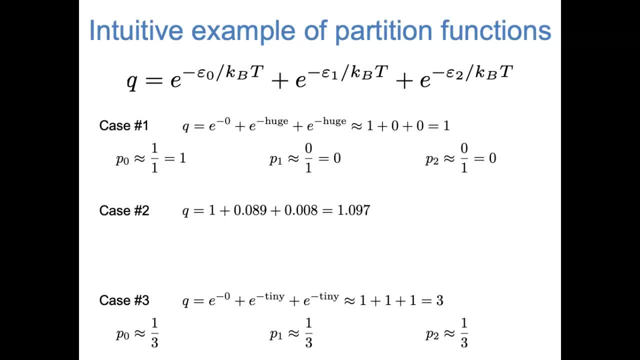 as the energy gets higher. You can check my math on this, but I got a partition function that's around 1.1, and if we want to find the probabilities of each state being occupied, we again take each Boltzmann factor and divide by the partition function. 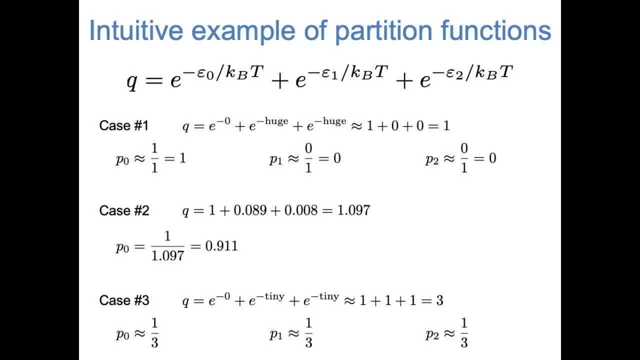 The probability that the ground state is occupied is one divided by the partition function, which is about 91%. so that makes sense. The ground state is the most likely to be occupied and the probabilities get smaller from there. Eight percent for the first excited state. 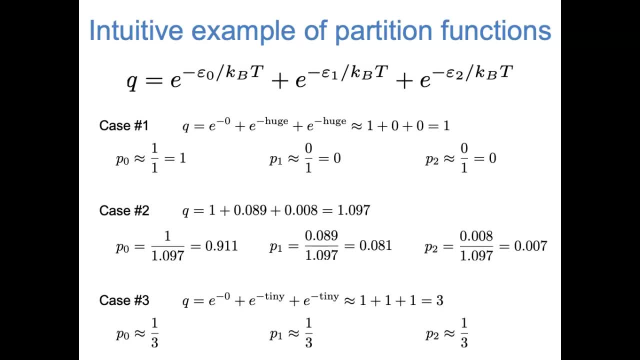 and less than one percent for the second excited state. There's one more thing I'd like to point out here. In case number one, where there's one state that's occupied, the partition function equals one. In case number three, where there are three states that are occupied, 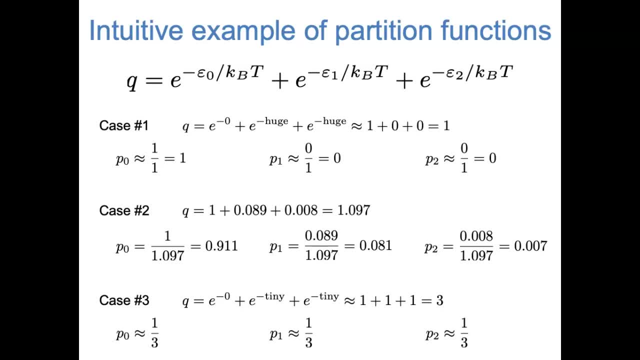 the partition function equals three, And in case number two, where mostly one state is occupied but a couple other states have some occupation, the partition function is a little bit more than one. That actually gives us an interesting, intuitive interpretation of the partition function. 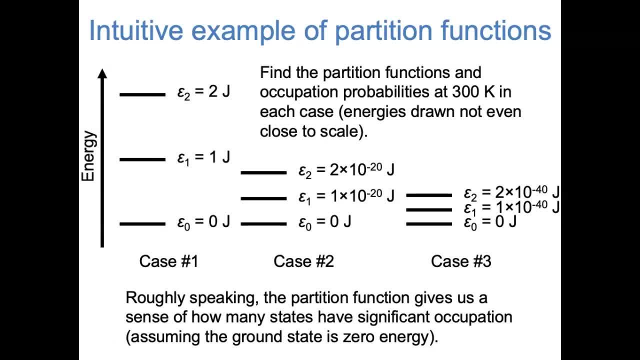 Roughly speaking, the partition function gives us a sense of about how many states have significant occupation, assuming the ground state energy is zero. Again, when just one state was occupied, the partition function approached one. When three states were equally occupied, the partition function approached three. 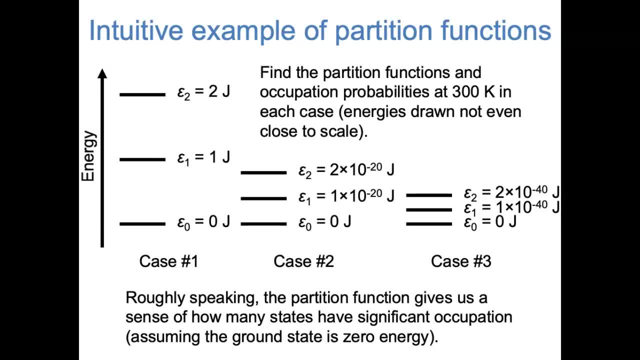 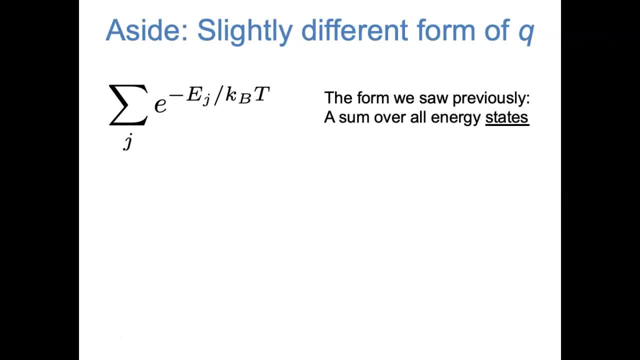 And when it was mostly one state but a little bit more in other states, the partition function was a little bit more than one. There's just one more thing I'd like to do in this video, and that's to introduce a slightly more compact form. 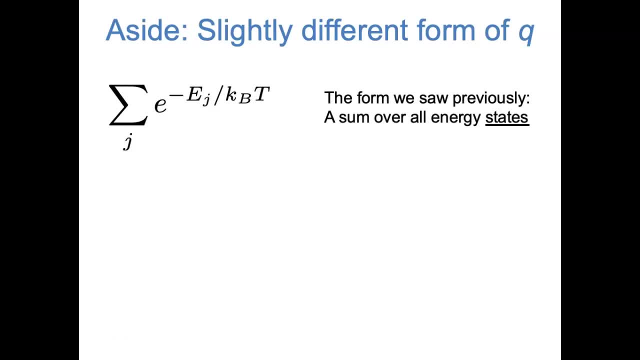 of the partition function. So far we've introduced the partition function as a sum over all energy states. We just take each state that the particle might be in and add together the Boltzmann factors for each of those states. In some cases, 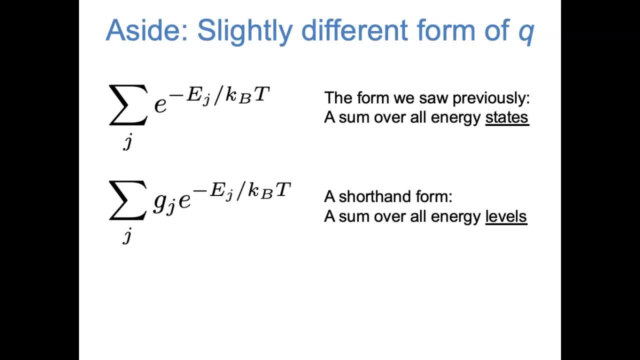 it would be helpful for us to talk not in terms of a sum over all energy states, but a sum over all energy levels, a sum over all energies at which there are any states. So this second form of the partition function looks very similar to the first. 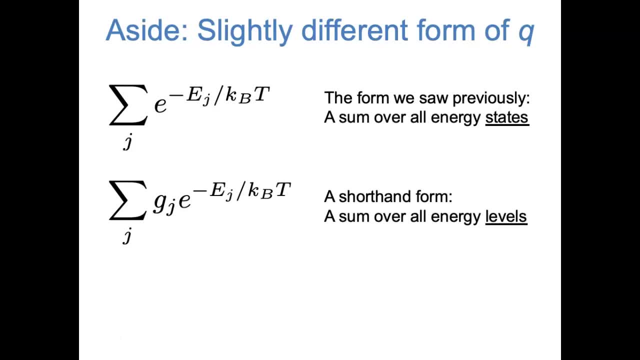 except that there's this extra term in here, g, with a subscript j, That's the degeneracy at a given energy level. In other words, if we have an energy at which there are three energy states rather than adding together the Boltzmann factor three times.